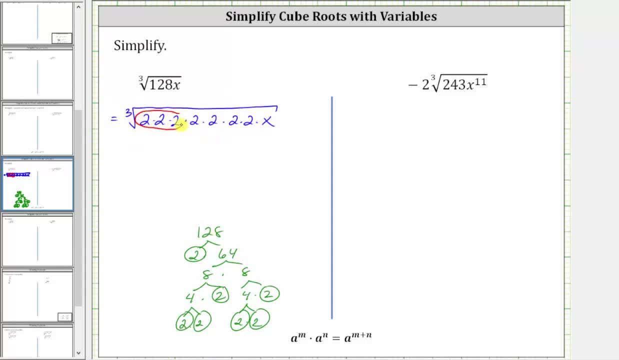 we know we have a perfect cube. Two times two times two is a perfect cube here as well as here, and therefore this will simplify The cube. root of two times two times two or two cubed is equal to one factor of two here. 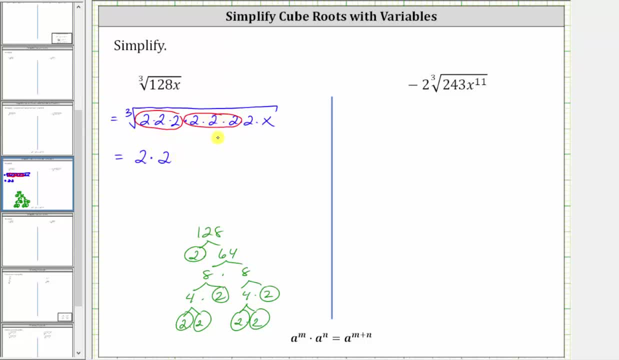 and then we get another factor of two here, and then we're left with the cube root of two times x, which is two x. The simplified expression is four times the cube root of two x. Next we have negative two times the cube root. 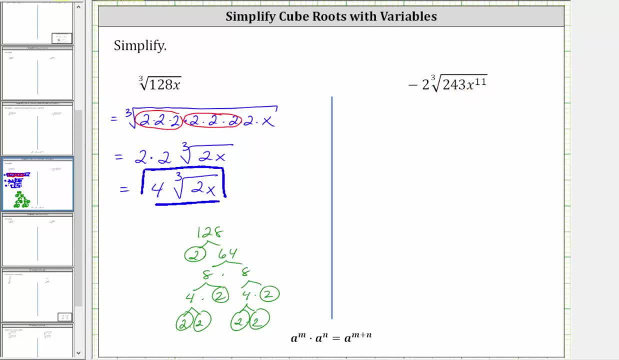 of 243 x to the 11th, To help us determine the perfect cubes of 243,. once again, let's determine the prime factorization of 243.. 243 is equal to three times 81.. If you have a hard time determining two factors of 243,, 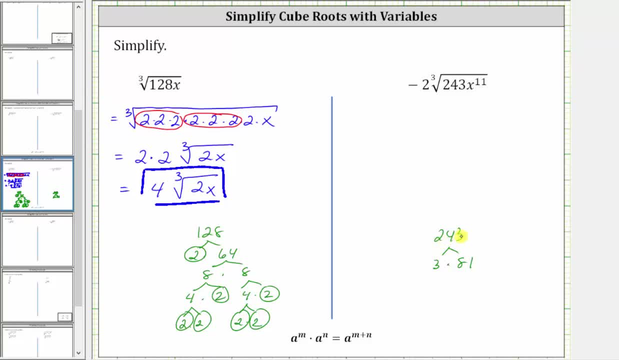 if we add the digits two plus four plus three is nine, because nine is divisible by three, so is 243.. And three is prime. 81 is equal to nine times nine, and nine is equal to three times three. Here as well as here, the prime factorization. 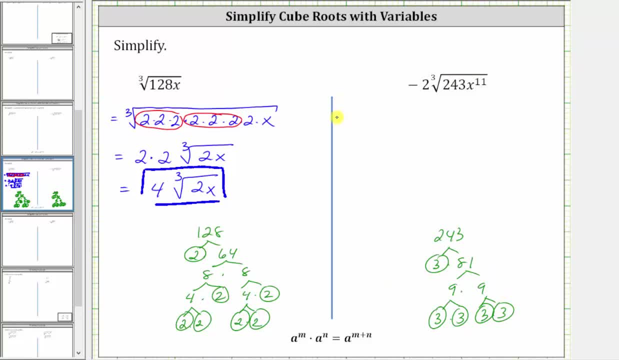 is five factors of three. Let's write the given expression as negative two times the cube root of five factors of three, And then we have x to the 11th. We know x to the third is a perfect cube. Let's see how many x to the thirds are in x to the 11th. 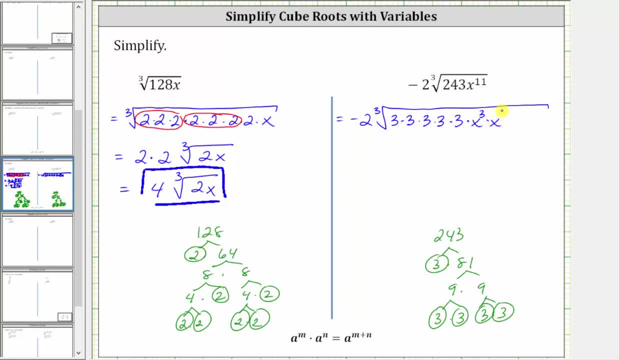 So if we have x to the third times x to the third, that would be six factors of x. Remember, when multiplying- and the base is the same- we add the exponents. If we multiply by another x to the third, that would be nine. 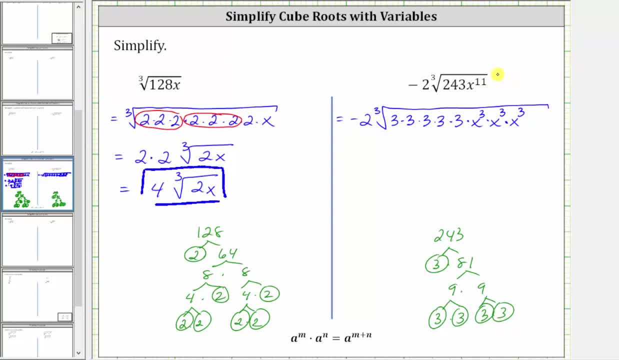 as we have nine factors of x and we have 11 factors of x, so we have two more factors of x and we're left with x squared. And now let's circle the perfect cubes Three times three times three is the perfect cube here.